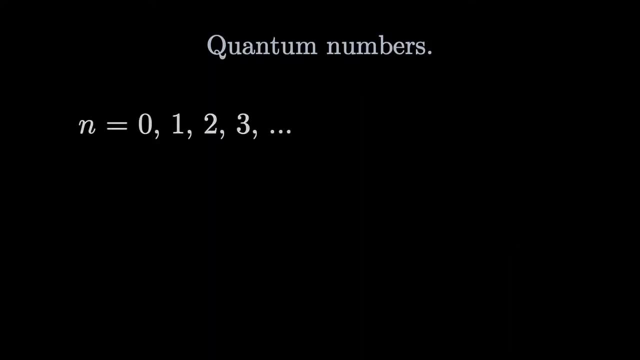 So it's that simple. The first quantum number is quite simple. Now our next quantum number is the quantum number l, And this can be from zero to n minus one. So, for instance, if we have n equals three, then l can be from zero to two, And if we have n equals four, then 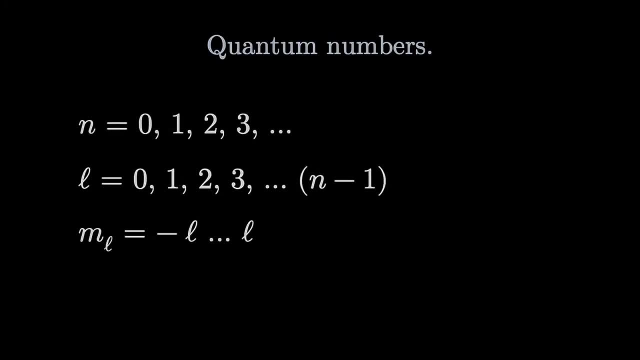 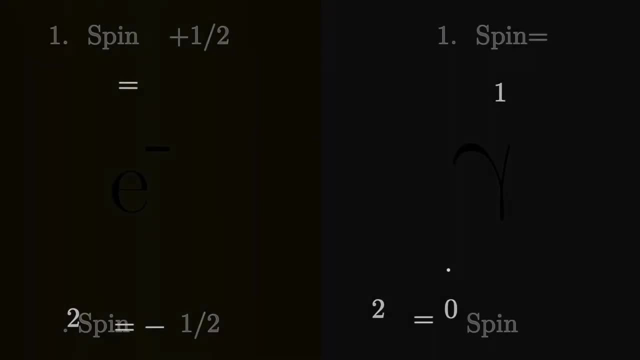 l can be from zero to three and so on. And our next quantum number is the magnetic quantum number, and this can be from negative l to l. And now the most important quantum number is ms, That's the spin quantum number In fermions. this can be either like positive. 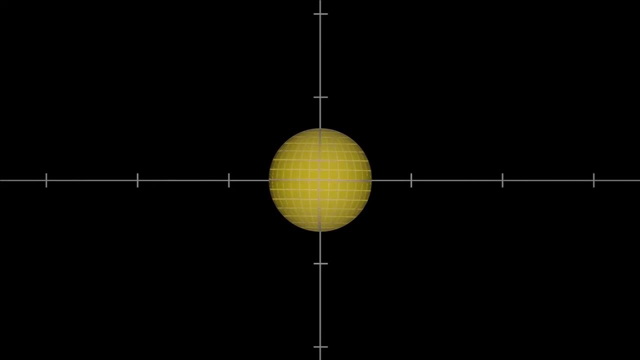 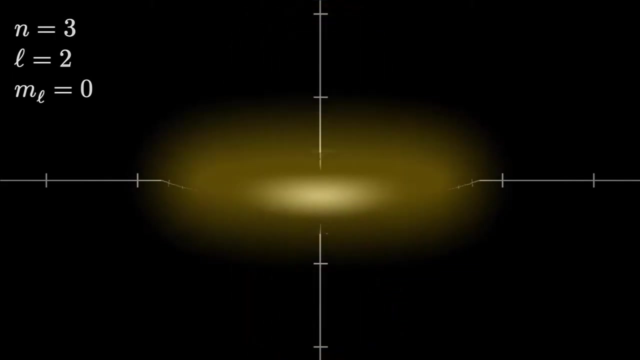 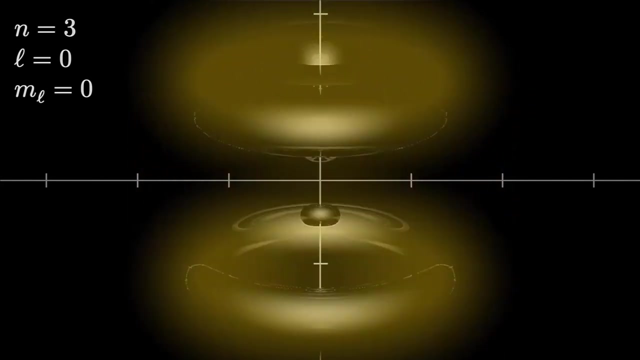 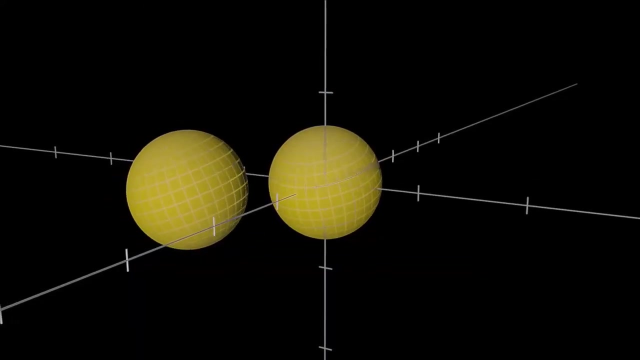 one and a half and negative one and a half, Although in a photon this is either one or zero. Now let's see how these quantum numbers changed the way the orbital looks. So since we built up a clear understanding on the concept of quantum numbers, let's talk. 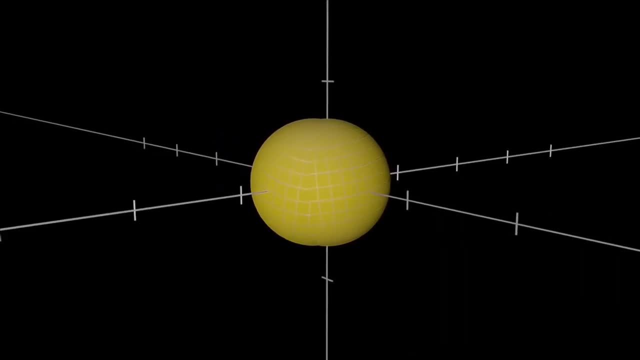 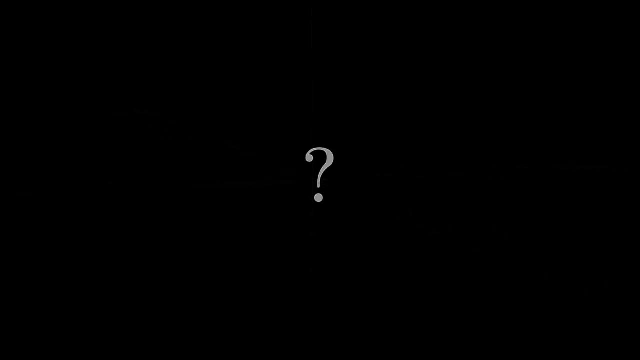 about the principle and what it claims. So this principle claims that no two fermions can share the same space and have the same quantum numbers. Since I called ms the most important quantum number ever, let's divide this into two spin eigenfunctions: alpha and beta. So let's start with an example. Imagine: 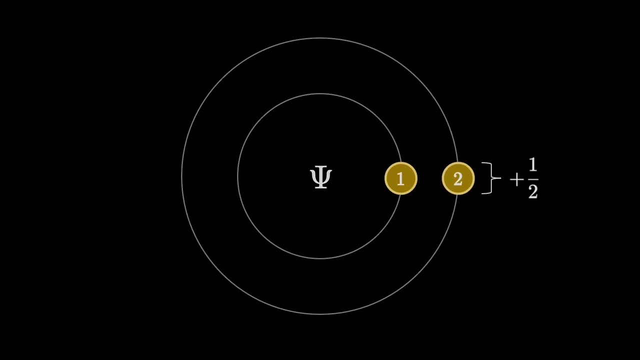 we have a system where we have two electrons and they both have a positive spin value, Then I can write this system as alpha one and alpha two, because alpha means the positive spin value. The good thing about this whole thing is, if we like, switch these up. The system didn't. 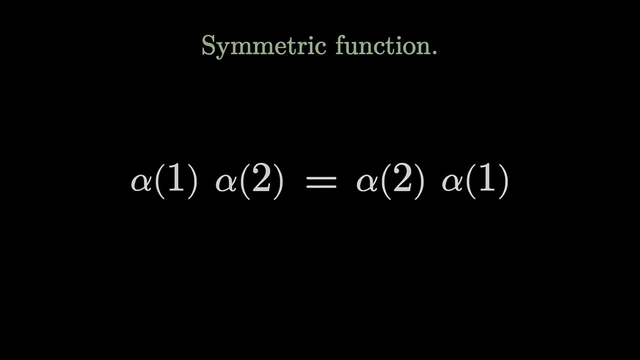 change. Therefore the whole thing is a symmetric function. So again, if they were like negative, I could have used the beta function for the electrons, as it can be seen here. So now let's talk about the spatial part of our function, Because at the moment our system 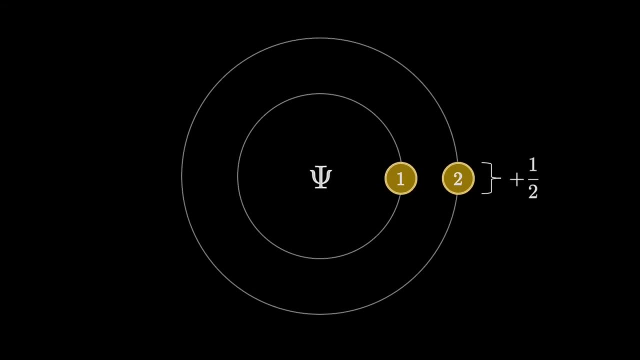 doesn't have any orbitals defined. So this is the system that we're looking for, Although at the moment we have just defined, This part doesn't have any orbitals defined. So this is the system that we're looking for. Although at the moment we have just defined this part, It's not going to change the orbit. It's going to change the orbit And the whole system is actually going to change. 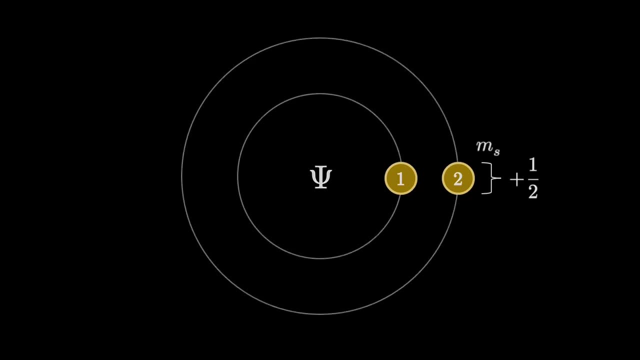 define this part of the system. So now we have to define the orbitals. So let's name the first orbital, psi A, and the second orbital, psi B, And the first electron is in the psi A orbital and the second electron is in the psi B orbital. So we can write them accordingly as following: 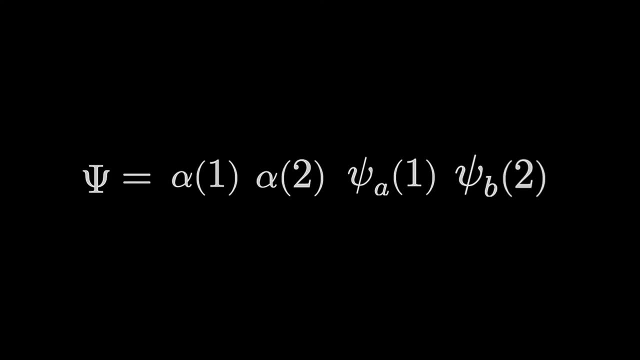 Now this is our whole system equation, So we have to pay attention to something. So this is the spatial part of our equation. If we flip these, we get the inverse function as it can be seen here, which means this function is anti-symmetric. 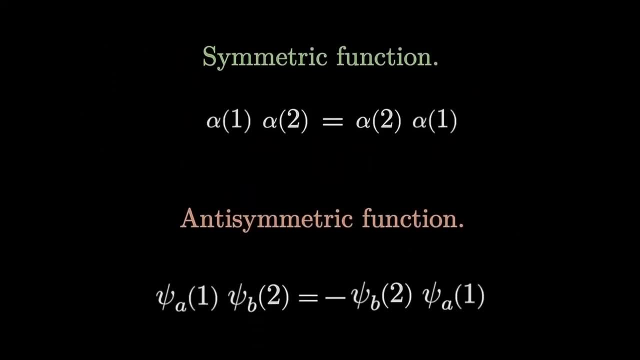 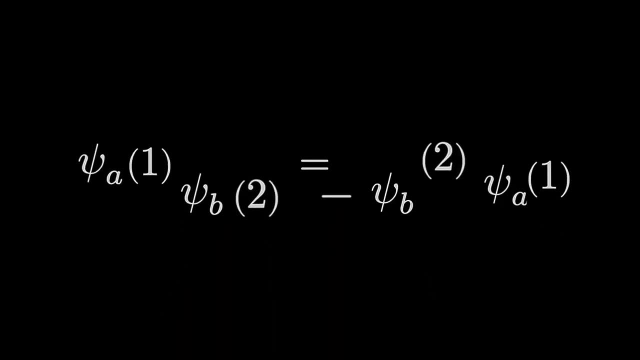 Which means our whole equation to describe the system is anti-symmetric, because if we combine a symmetric and an anti-symmetric function, our whole function becomes anti-symmetric. So now let's use the superposition principle and we can erase the equal sign. 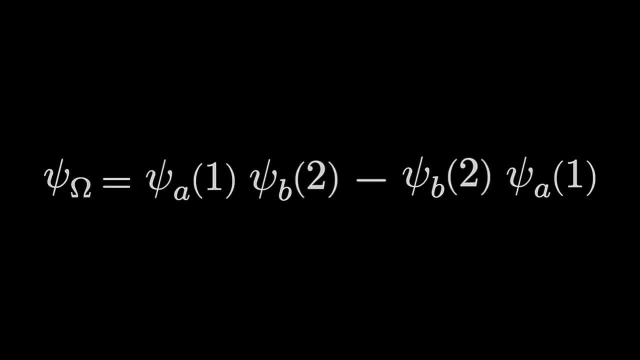 Now, this is our spatial part. I will make a video about this principle later, although now let us accept it. So this is the spatial part of our equation and these are the spin values of our equation. So if we combine them under the whole system equation, we get this: 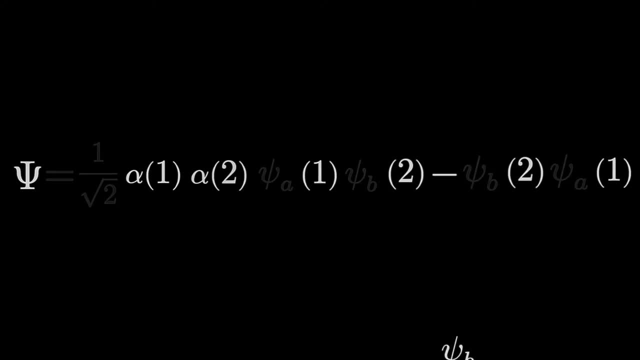 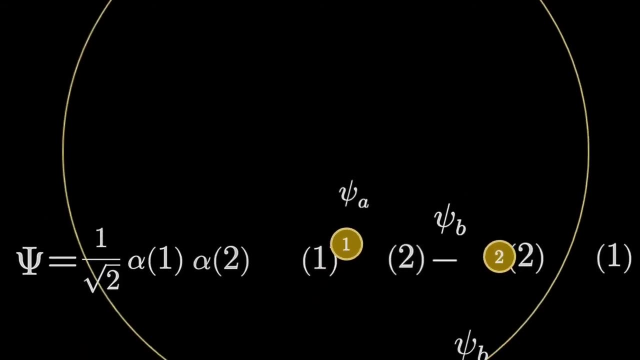 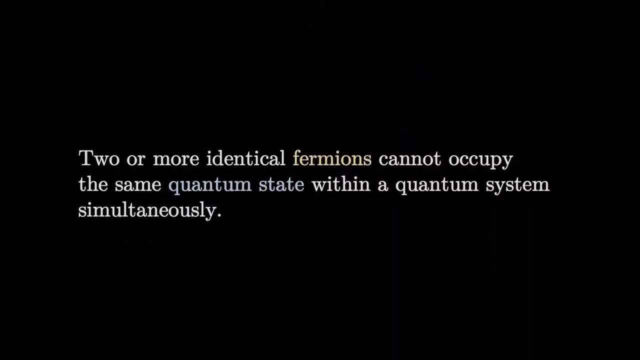 Although, before I put the equal sign, we have to normalize this whole equation by putting this: 1 divided by square root of 2.. I will also make a video about this. Why So? at the moment, this whole equation describes this system. So, in order to test this principle, let's return back to the definition. 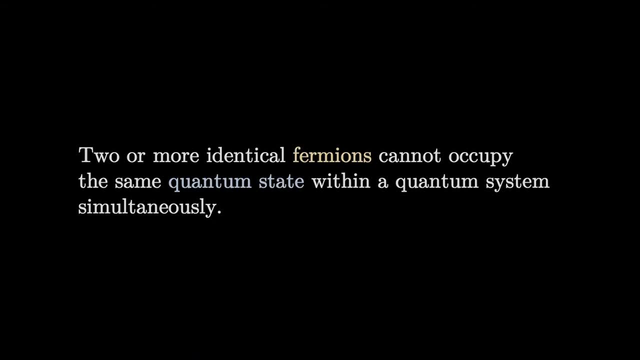 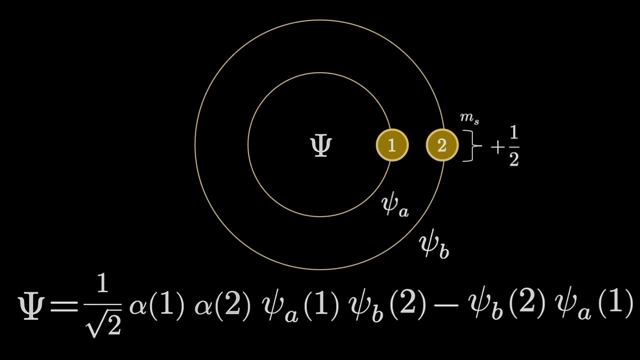 Two or more identical fermions cannot occupy the same quantum state within a quantum system simultaneously, So we have to make these electrons share the same space, And in order to do that, we can make the orbitals approach each other as the following, And this is what happens. 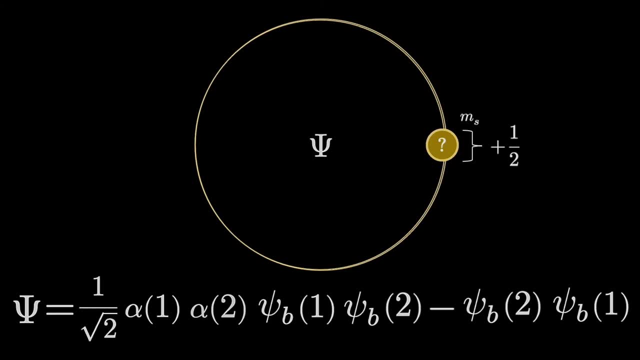 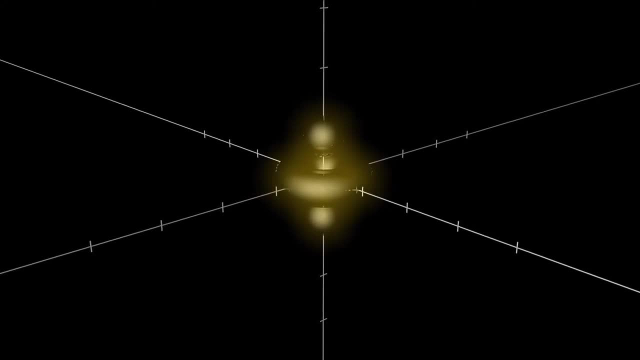 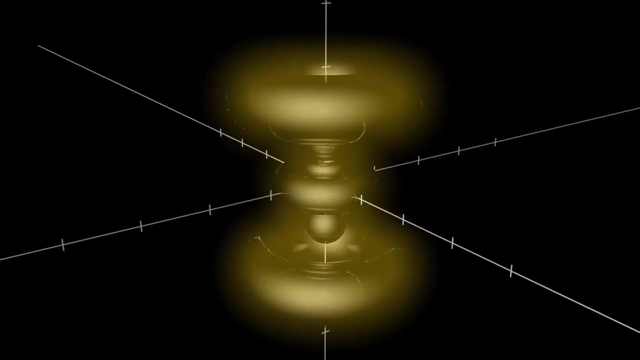 in our equation, if we do that. So let us like visualize this whole thing in three dimensions. So imagine this is our first electron that we have in the first orbital. Now let us define the second electron that we have in the second orbital. So now we will be making the side A orbits approach the side B orbits. And when we do that,